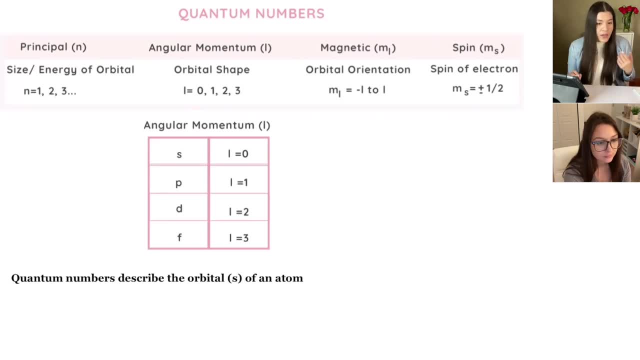 already with like n, with electron configuration where you had like 1s, 2s and so on, and we were talking about the energy of the orbital. So n really just describes the size or the energy of the orbital And we know the higher up or the higher number it is, the more energy it has. 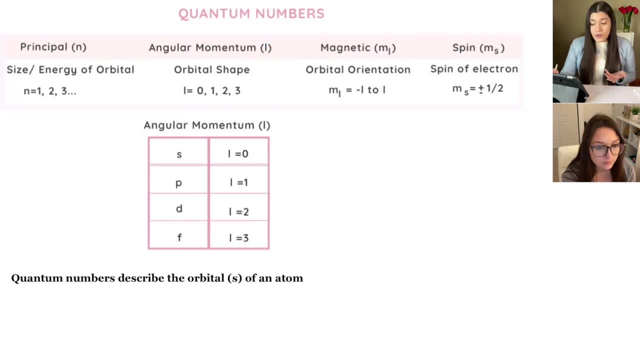 And then versus the next one, which is l or angular momentum. that just means like, what shape is it? Is it s, Is it p, Is it d or f? And remember those shapes that we were looking at before, like s had more of a sphere shape right, And then p had more of that, like kind of like a balloon. 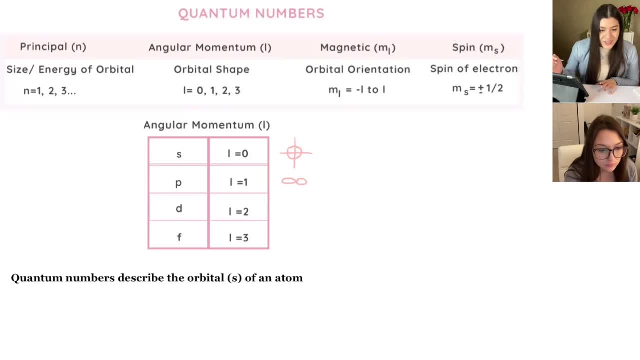 where it looks something like that right, Kind of like those like balloon animals, it kind of looks something like that. And then c and then d and f were a little bit more, I'd say, more complex. You're not expected to know like the shapes of, I'd say, even f or d, but that's basically just describing the shape for the next. 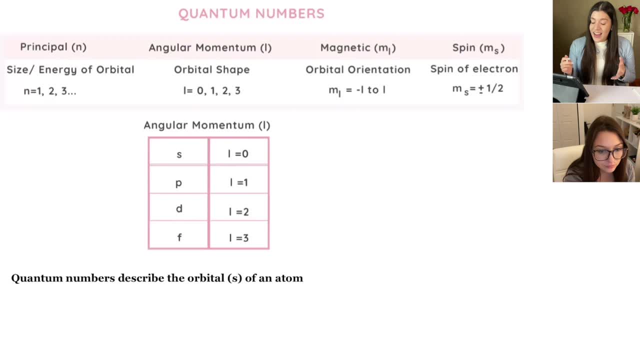 one. Now it's going to be really important to understand. actually have this memorized. So you're not going to get this on the test. Definitely have this little table here memorized completely. So if l is equal to 0, it's going to be s, If l is equal to 1, that's going to 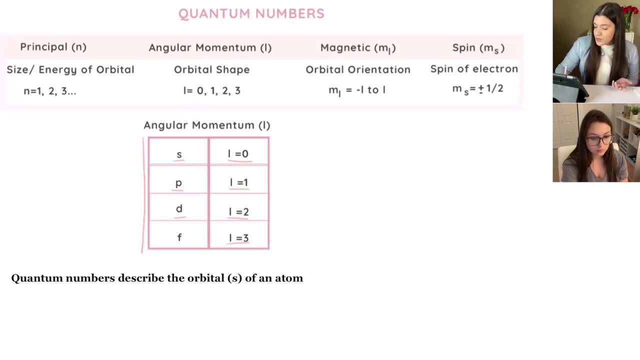 give us: p? l is equal to 2.. d? l is equal to 3 f. So instead of it being like 1 through 4, it starts 1 less, So it starts from 0 and then goes to 3.. And then now for the next one, that's basically. 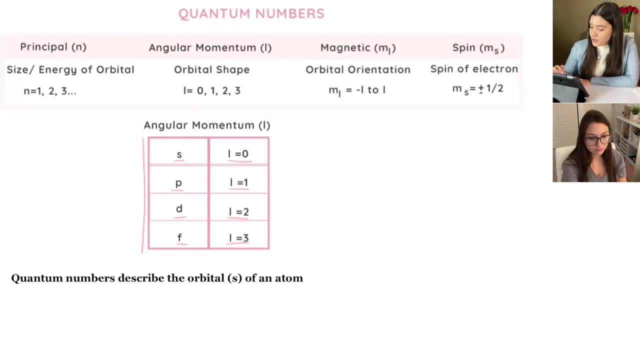 just going to tell us the orientation of the orbital. So you can think of it kind of like with p, how this is centered on the x-axis or y or z-axis, and it's basically telling us where is it So how is it Oriented. So this is going to be really important to know because, like you have to know the l to 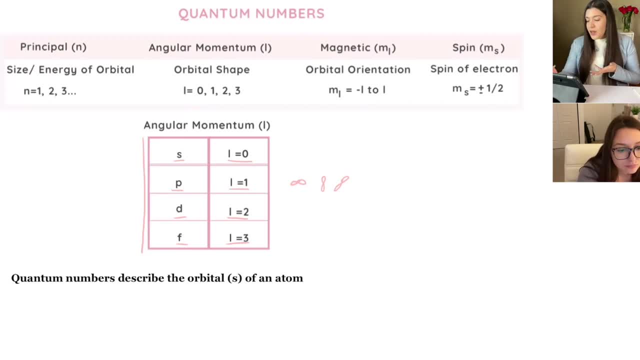 know the m sub l or the next quantum number. So m sub l is basically just the negative l to the positive l, and I'll explain what this means. So if l is equal to 1, then that means the m sub l is equal to negative 1, the next number, 0 to positive 1.. Like if this was 2. 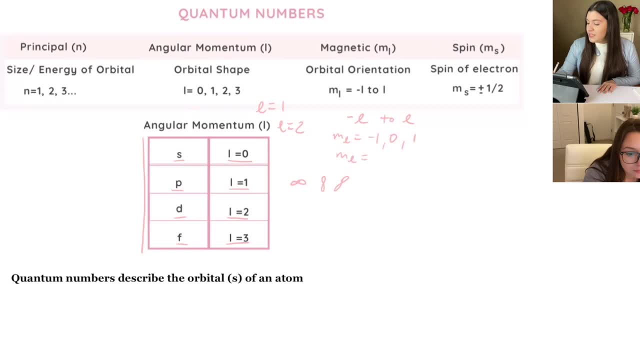 if l is equal to 2, then m sub l is equal to negative 2.. Then all the numbers in between, all the way to positive 2.. So next one is negative 1, 0, positive 1 and then positive 2.. Does that make sense? Actually, no, I'm confused, I'm sorry. Okay, no problem, What doesn't make? 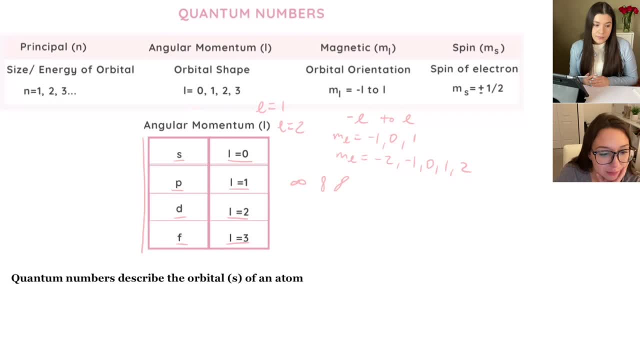 sense. So okay, so I get that l represents these different things. but what is the m sub l? It's the orientation of the orbital. So, like, like for the p orbital, there are different, like there's three of them, or I'd say, actually, like this is px because it's centered on the x-axis. 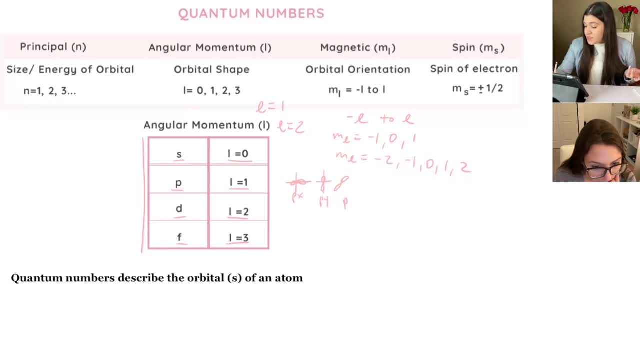 This is py because it's on the y-axis, and then this is pz because it's on the z-axis. So it's basically just like: how is it oriented in space? Okay, Does that make sense? Yes, So are they gonna like ask us to write out? 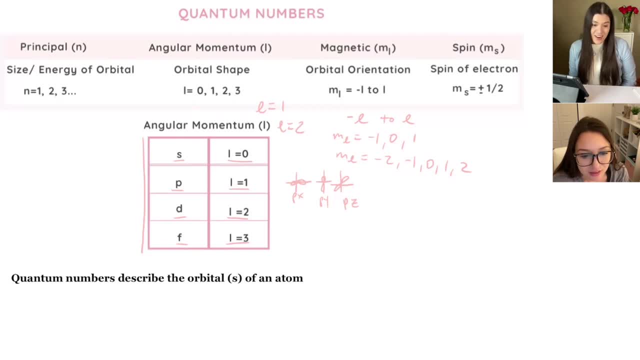 Like negative 2, negative 1? Yes, Yes they are. They're gonna ask you like to actually write out all the possible quantum numbers for an atom or for a specific atom. So we'll definitely have plenty of practice of this. but just knowing that it's always that from that negative l value all. 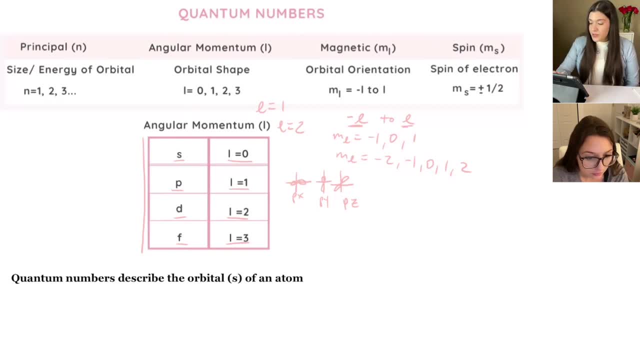 the way, like all the numbers in between, to the positive l value, So like when l was equal to 1. I start off with the negative value. so negative 1, the number in between 0 and then the last one is just the positive value. Okay, I get it now. The first time you said it, I like didn't. 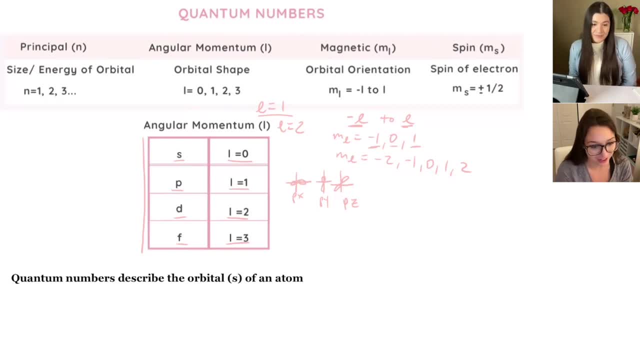 understand like what that, where that was coming from? Okay, that makes sense. So that's why we have to memorize the initials, so that we can do it. Okay, got it. Yes, perfect. And then the last thing. so everything we just talked about talked about the orbital, The m sub s or the spin quantum number. 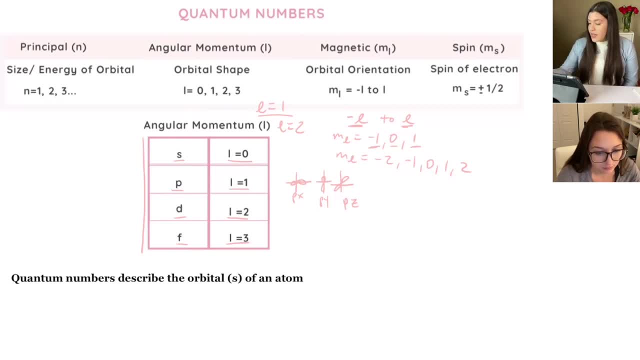 talks about the spin of the electron. So remember, that's kind of like what we saw before when we were doing orbital diagrams with our electron. So we're going to talk about the spin of the electron, Showing the spin like, oh, this is going up. Well, that's a positive, That's a positive one half. 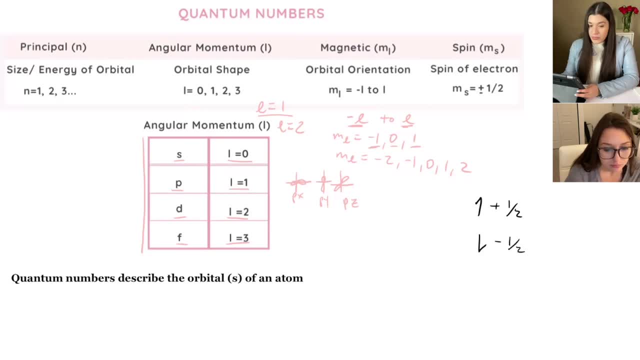 And then if this is going down, that's a negative one half. And then if we were to have like, let's say, that little orbital diagram that we saw before, Let's say this is 1 s 2. Well, we saw that this filled that orbital, And then I know that, okay, well, this is both plus or minus one. 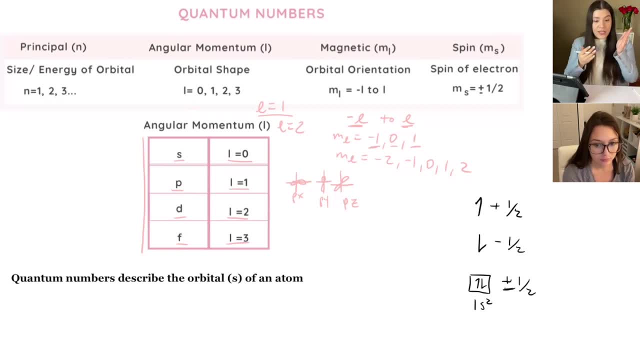 half, Since I have both the- you know, the positive one and the negative one- pointing down Cool Questions here so far. No, it makes sense. Yeah, I'm glad because I was doing these. these I've already covered like in the homework, But I did not understand it. 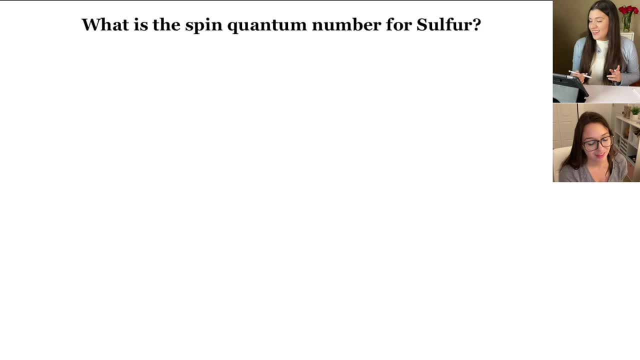 Like I didn't get it, So now I get it, Got it, Okay, nice. The next thing I'm going to look at right now- I'd say this question isn't as common. The next ones that we will go, after this one over. 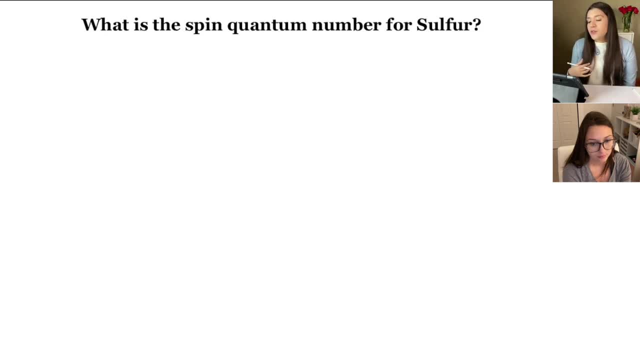 like those are going to be the most common, But just in case they throw it. So for this, this is saying: what is the spin quantum number for sulfur? Remember, the spin quantum number was the one we just saw before, Which was that m sub s And that. 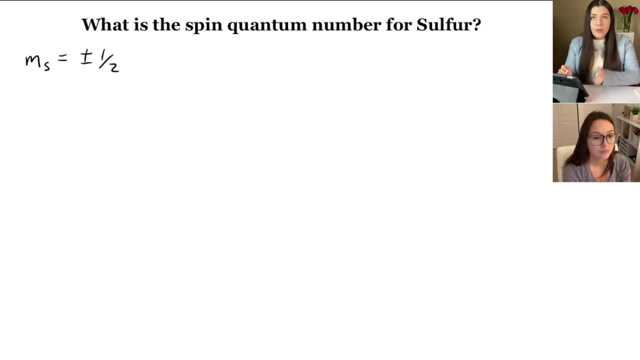 could either be plus or minus one half. Now, how you could figure that out, Like how do I know if it's going to be a positive one half or a negative one half? That's going to be based on our electron configuration of the atom that they give us, Which in this case is sulfur. So let's kind of go back. 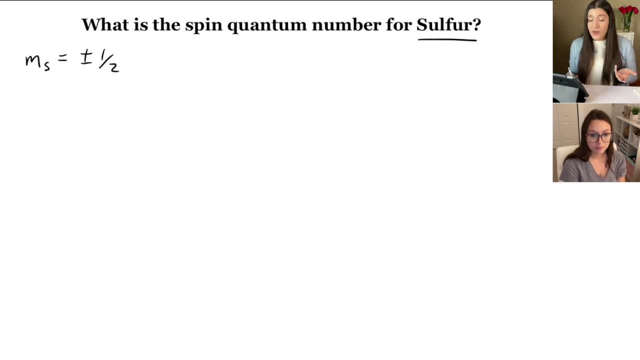 to what we learned before And write out what the electron configuration is for sulfur. You could just do the abbreviated or Condensed electron configuration. Do you have your periodic table on a needle? Okay, By the way, Side note, I got, I took all of your things and I put them in clear things and I'm I. 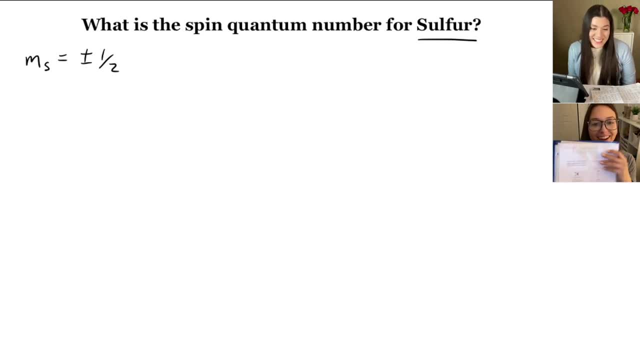 need to get a folder with like things in it, But I'm going to put it in there and I have all of them, So it's like so cool, And then I put in the front like periodic table. Very nice, It looks really nice. 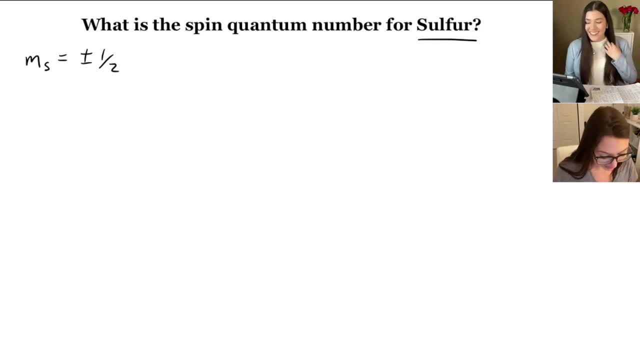 Thanks, I'm like so happy about it, Okay Anyway. So sulfur, Here we go. Let me figure out where that is On here. Okay So, it's going to be neon In the brackets And then 3s2.. 3p4.. 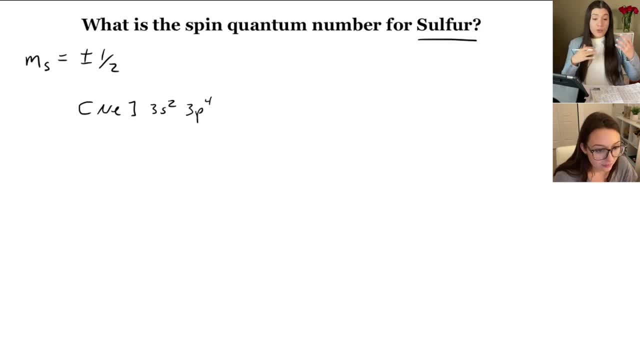 Correct, Perfect. So now, if I were to draw the orbital diagram of this, So I'll do that now. So we know, will represent just, You know, make that nicer. Our first one, which is 3s2.. And the next one: 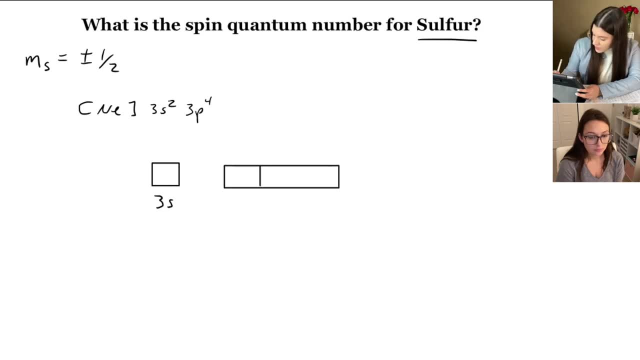 We need three, Since this is going to be 3p, And then I'll do What we did before with our orbital diagram: ther's 2 electrons here And then. now I want to look at those 4.. Obeying Hunt's rule. 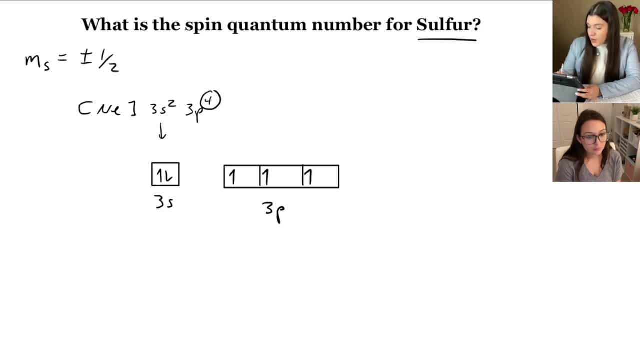 So this is one, two, three- come back around- and four. So this question is only looking at the last electron. So is it, you know, pointing up? Is it pointing down? So our last electron was this: And since that's pointing down, our m sub s is actually a negative one, half. 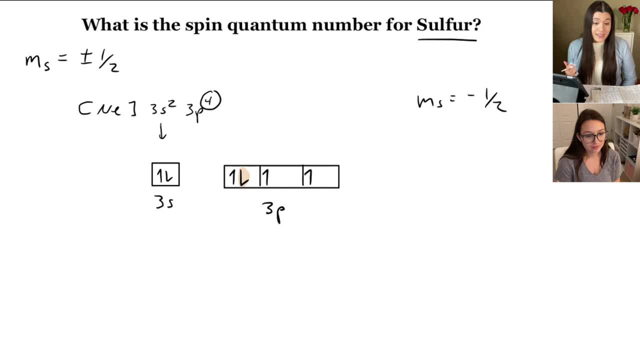 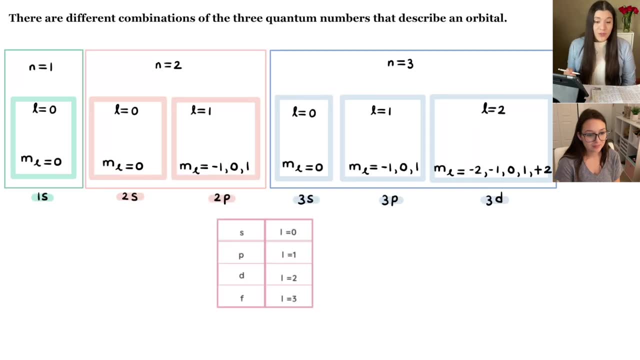 Okay, that makes sense. Cool, That's it. That's how you would answer these types of questions. Cool, That's not bad at all. Awesome, Okay, moving on. So, like we said before, the first three quantum numbers, so like n, l and m sub l, describe what our orbital is. 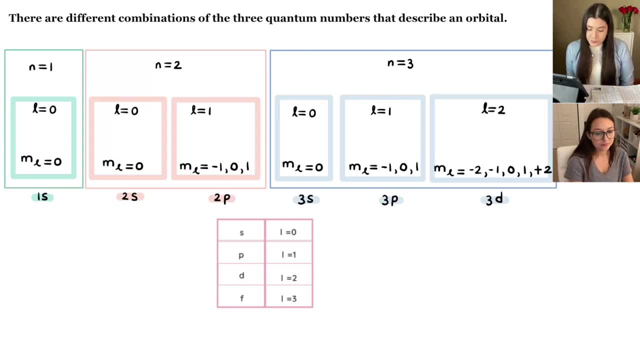 essentially going to look like the energy level and so on. So I wanted to explain a little bit more where this comes from and how everything comes together. So starting off with, let's say, something that is in that like one s category, So in that first row, 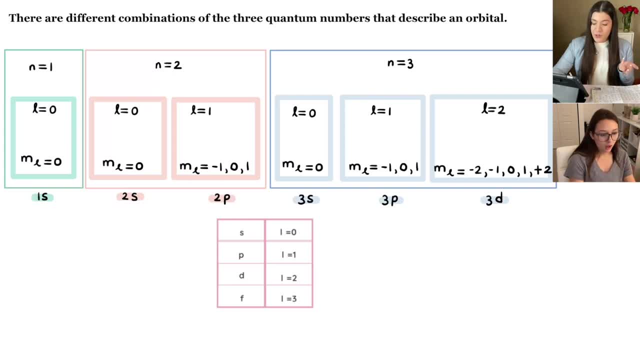 on our periodic table. we know that well, that one is actually going to represent our n, or the energy of our orbital, And then the l that comes from our little chart that we saw before, which is going to be the shape of the orbital. So l is going to, since it's equal to zero, 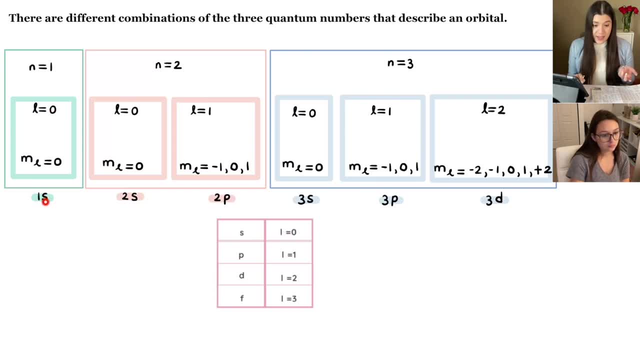 that means it's s. So that's where I got. okay, I know that's s. And then the last thing again was m sub l is equal to that, negative l to positive L, And since l is only zero, we can't have a negative. you know about, there's no negative. 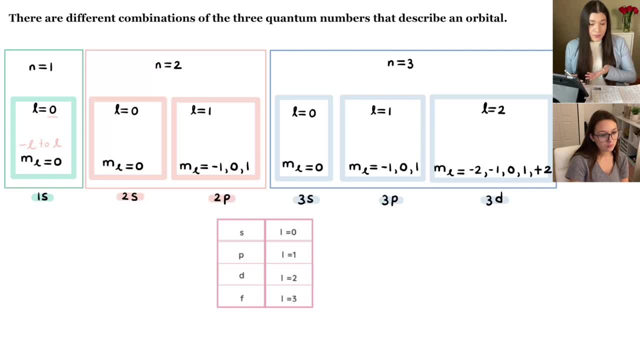 zero, it's just zero. That's why m sub l is just zero. Does this make sense? Yes, I'm just like trying to figure out how that's going to apply to a question. You know what I mean. So, like, what are they going to ask me from this? 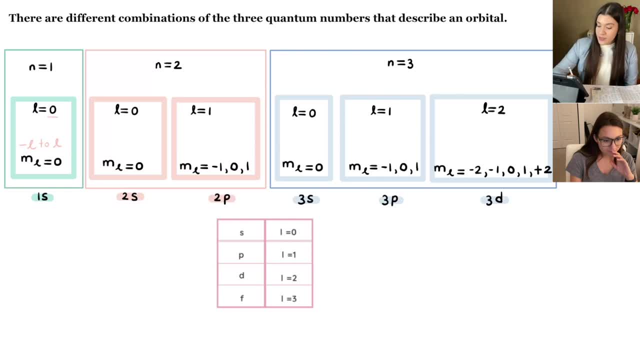 So you could actually be asked like you can just be given one s and they'll ask you write all the possible quantum numbers, And then you'd have to know. well, okay, this one tells me the n value, which is one. This s represents the l value here. 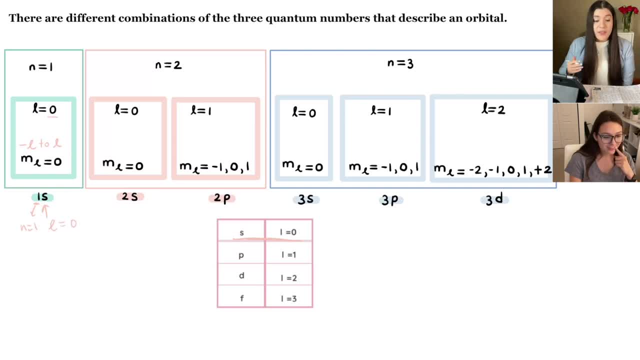 So I know l is equal to zero. And then from there, since I know m sub l is like that negative one to sorry, that negative l to positive l, then okay, m sub l is just zero. So do you think I need to know which thing represents, like which one's the shape? 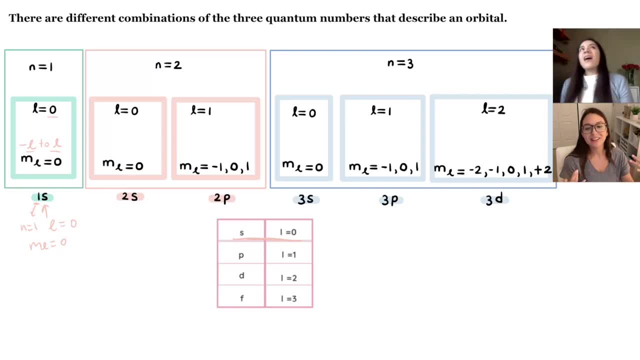 which one's the spin, or whatever. Yes, Because they might- At some point, Exactly, Exactly. They might ask it in a question and they won't say, oh, what's m sub l, They might say, oh, what's the orbital orientation You know? and if you don't know that, then 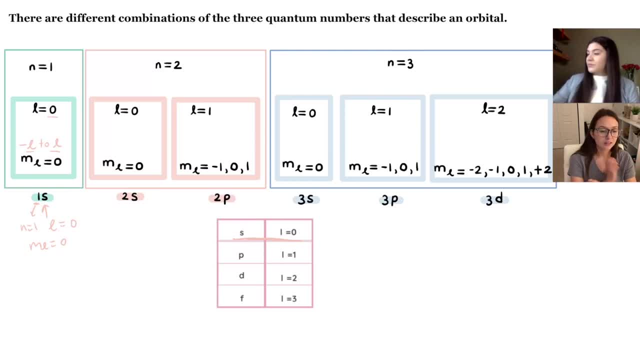 you know that doesn't help. Okay, got it, And then same goes for the next part. So what we could actually be given in this case was we could just be given: well, n is equal to two and then l is equal to zero. 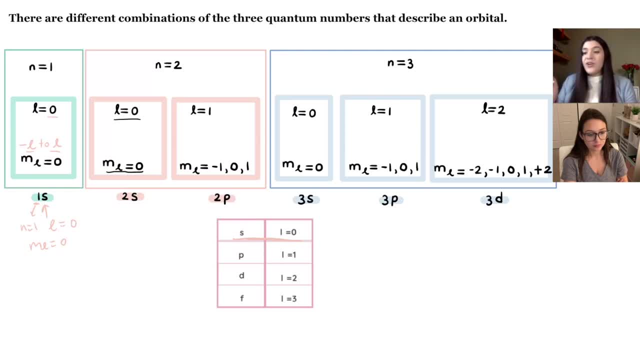 and m sub l is equal to zero, And we'd have to figure, figure out what the like, the orbital is essentially. So if they were to ask that, then we know well, two is going to represent the coefficient in front, And then I know l is. 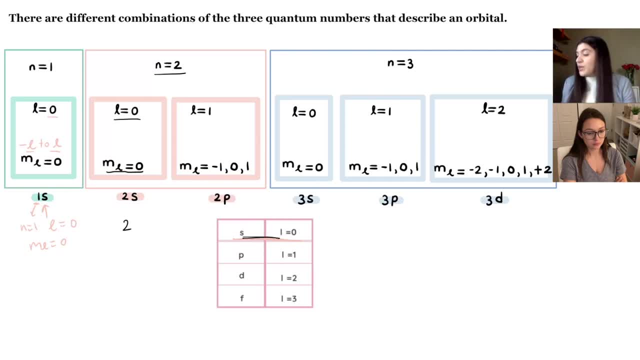 basically telling me exactly what orbital shape it is, so zero or, sorry, s, And then I know that's where this came from. So two s done. I don't necessarily need the m sub l in that case, But that's another way. So it could like either way doesn't matter, You could figure it out. 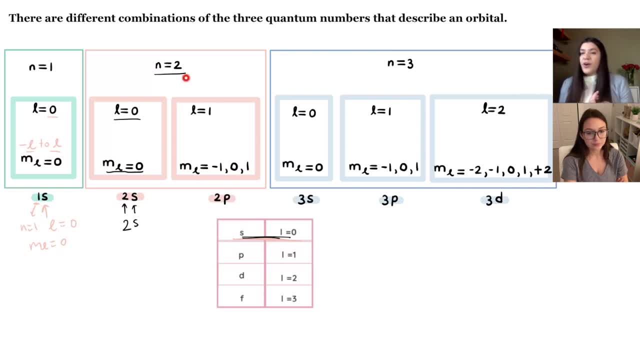 I'm going to kind of jump to this, This end here. So same thing for this part. I know that, like if I were to be given to p, the n is going to be two And then p. we know that this would have been. l is equal to one. 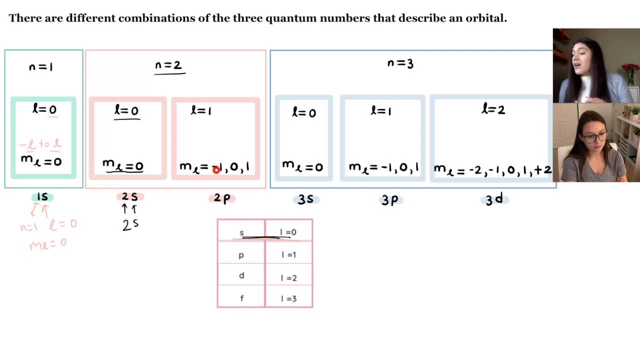 Our m sub l is our negative l to positive l. So negative, one, zero and one. Next one here. If I were to have three s, I know that my n is this value in front, so three If it's s. 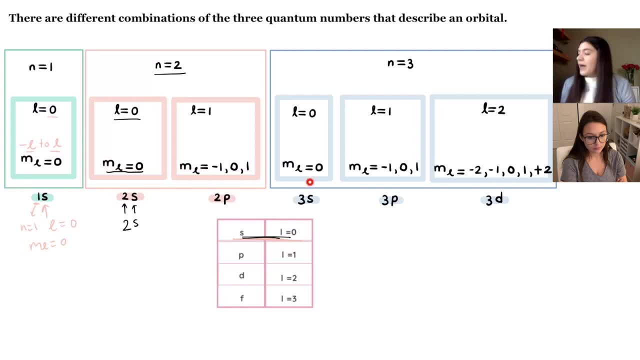 that's going to give me zero For my l, And then m sub l is zero And you're going to keep seeing this pattern Like, okay, three p? well, like the n I'd say is probably the easiest one to identify. And then, where most, 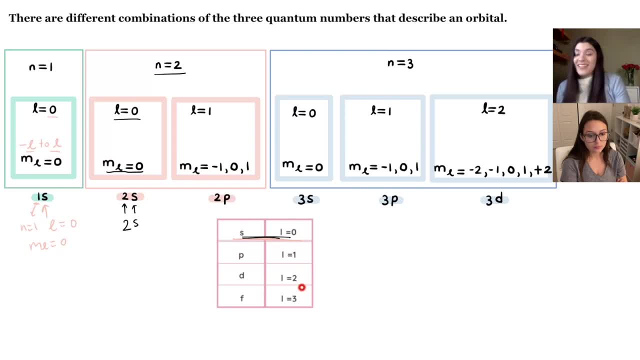 students go wrong is just forgetting this table. Okay, so this, like the fact I know, is it's sometimes like something extra that you have to memorize and you have more than enough to memorize. I remember So that p just knowing- okay, well, it starts off from l- equals zero. 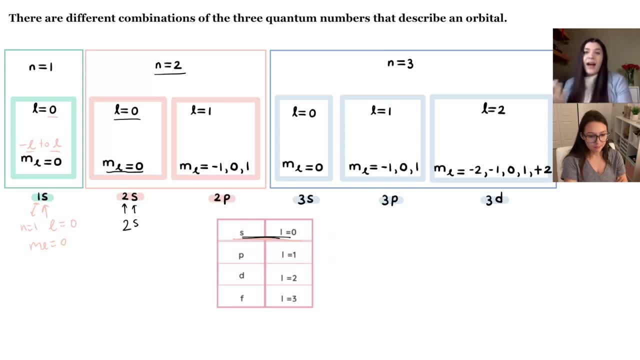 l equals, one is the next one And p is the next. like higher orbital energy, I guess I'd say higher up in energy. So that would be p And we'd go from there. So any questions so far. I want to do a bunch of examples. 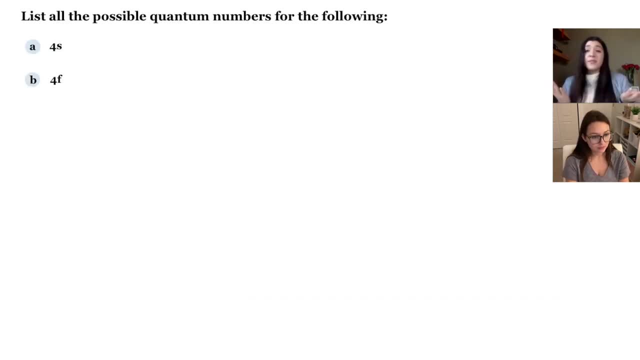 No, it makes sense. I'm good. Thank you For this one. this is a potential question that they could give you saying: list all the possible quantum numbers for the following. So I would start off with a and I'll see well if this is. 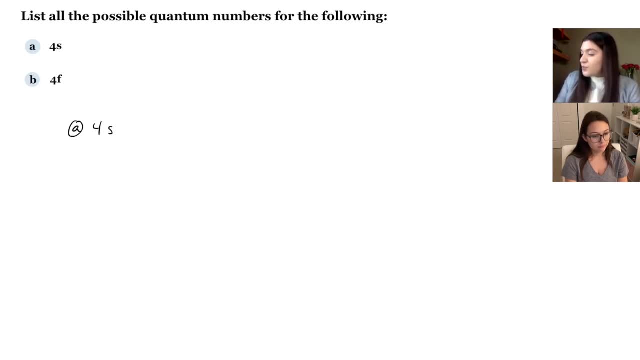 four s. this first part is telling me what the n value is, So n is equal to four. And then next the s tells me what the l value is. So remember that table, the first one, l equals zero, is our s. 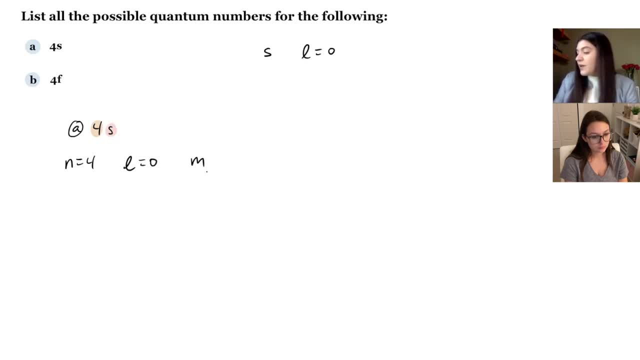 orbital. So that would have been just zero, And sub l then would have been basically just negative l to positive l, which in this case the only thing we could have is zero. So that's what it tells me And the last one m sub s there's nothing like. there's no other information. 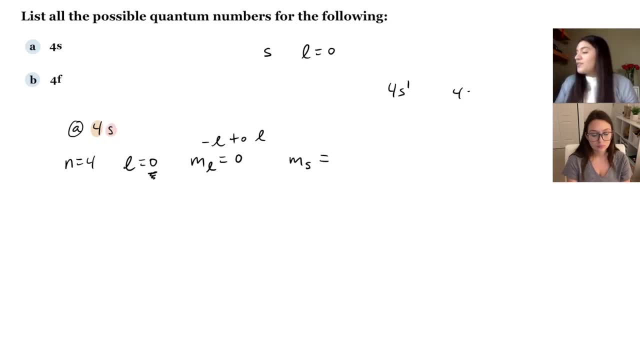 Like this doesn't tell me that it's four s one or four s two. It just says four s. So I'm just going to say it's plus or minus one half. However, if this were to have been like four s one, 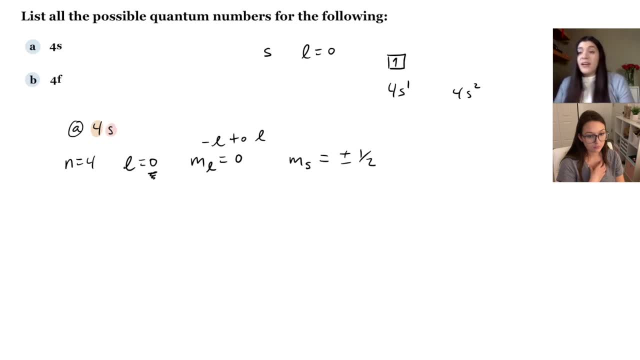 remember it would have looked something like this: where it's just one electron there, So that would have been pointing up, So that would have been a positive one half. But if this was four s two, then I would have two electrons, And I'm just focused on that last electron And it's pointing. 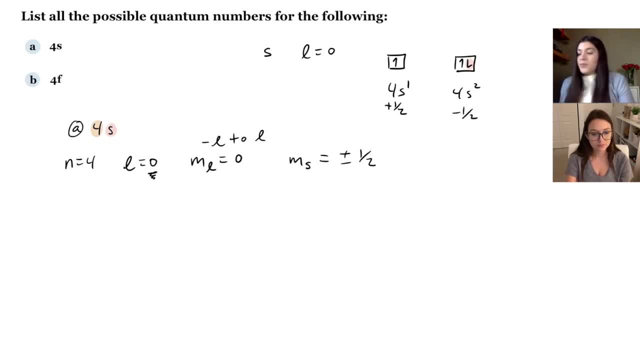 down. Okay, But because they don't tell me, I'm just going to say plus or minus one half, And then for part b a little bit different. So now we have four f Again. this four is going to represent our n And then our l. well, this is, I know. I'm going to figure out the l from the. 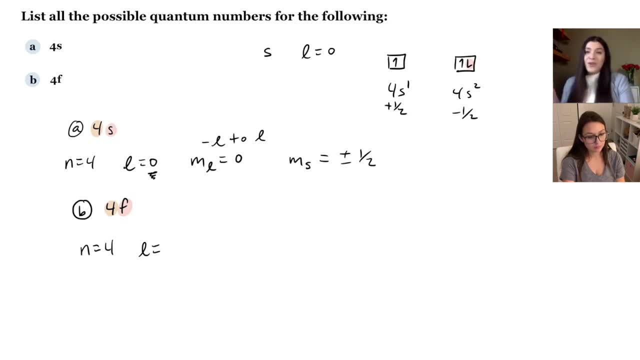 whatever like value I have here. Sorry, whatever orbital I have here. So I have f. Remember. the table looks like this: where there's s, then there's p, That's one, d is next, which is two, And then f is three. So I know l is going to equal three. I'll move on to the next. 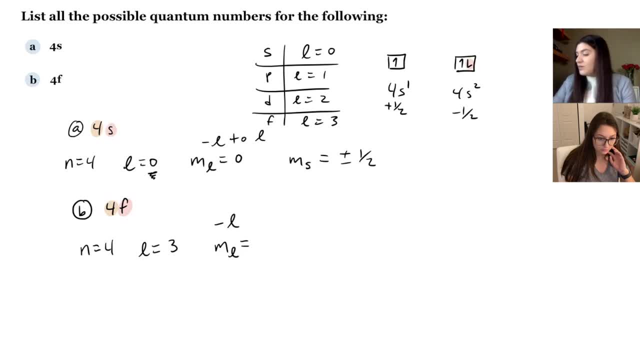 quantum number m sub l. So this is a negative l to positive l. So I'll start off with the negative l value, which is negative three, Then continue with all the numbers in between. So negative two, negative one, zero one. 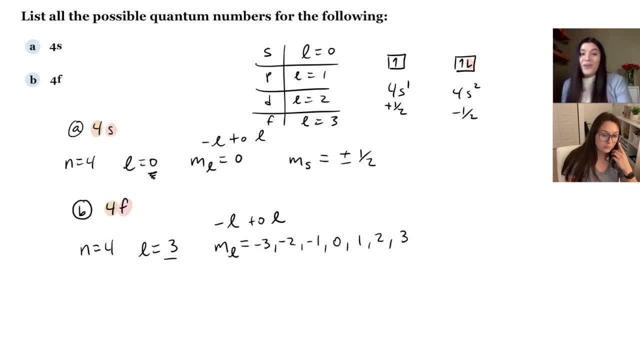 And then two, and then to positive three. So all of those values are possible. And then the last thing is just that spin of the electron, or m sub s. Since we don't know, I'm just going to say plus or minus one half, since they didn't specify how many electrons. 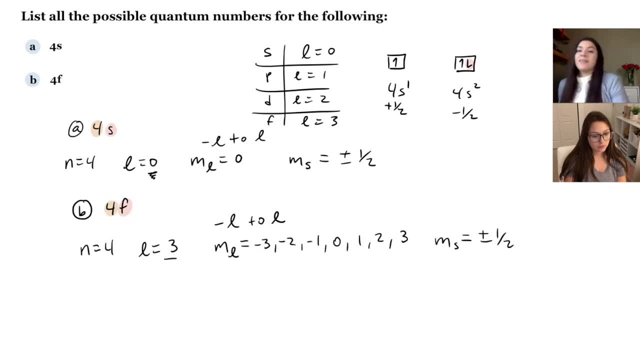 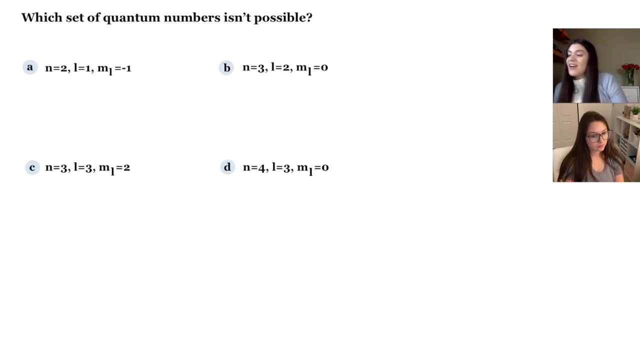 are in there Makes sense. Yes, Cool. Okay, This next one, All right. So this question I have seen on most exams. Definitely know this. This one is. it may seem tricky at first, but I'll explain it. I'll help. 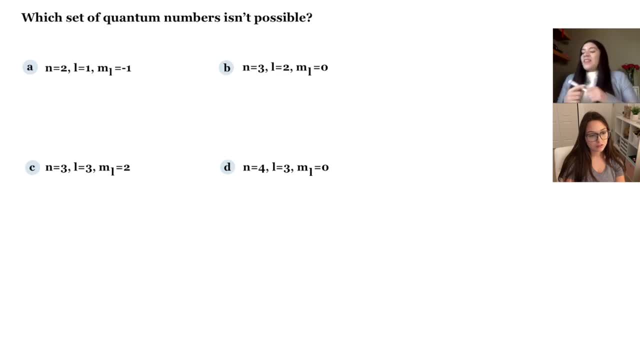 you understand it a bit better. So this, basically, is telling us which set of quantum numbers isn't possible, And we're going to go through every single one and I'll tell you why it either is possible or isn't possible. So, starting with the first one, just looking at a, I want you to 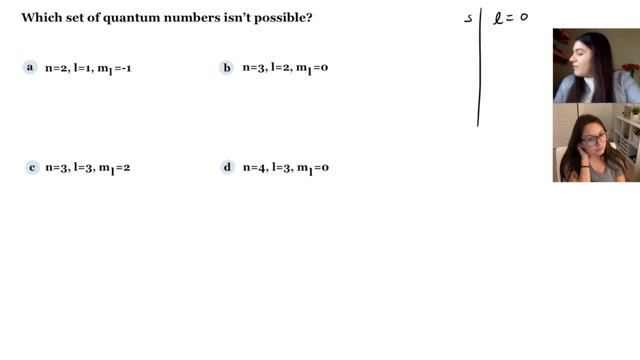 and actually I'll write out what we have here for that table. No, you don't have it memorized just yet, since I literally just taught it a second ago. All right, So just looking at a, what does this represent? And by that I mean like 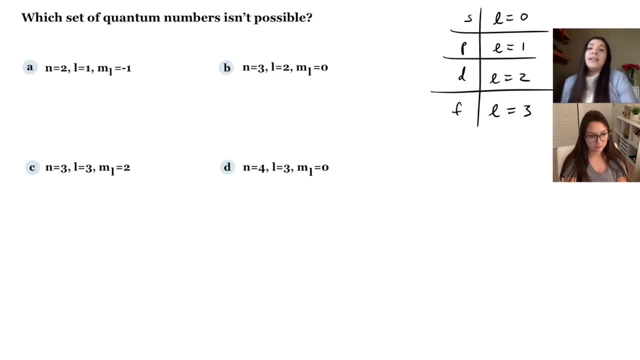 is it one s, Is it two d Or two p? You know what is it? Oh, it's um two s. Try that again. So you're right with the two Oh, two p, because it's a one. 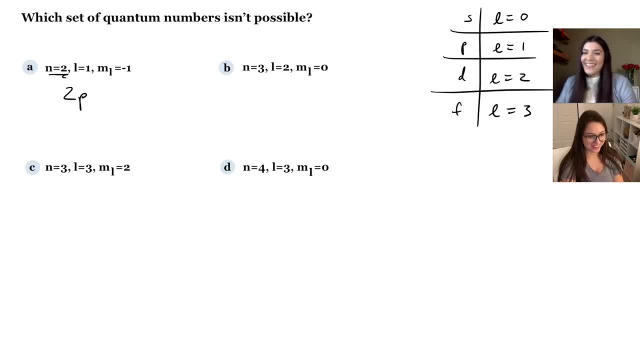 Yes, Okay, Wow, I didn't know you could go backwards with this. Okay, Two p, And then that's all we would know, because this doesn't tell us you know what, what, anything else, Like we don't know how many electrons there are, It just tells us, okay. 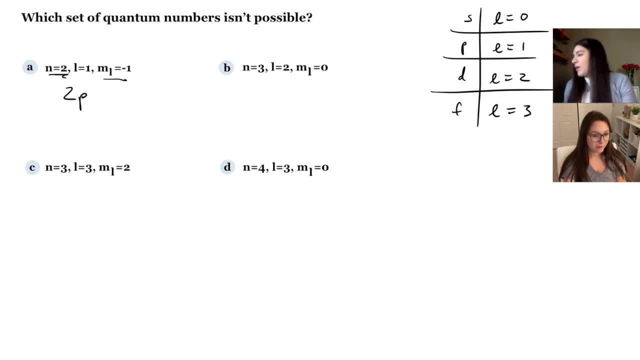 this is two p. Well, I know that, looking on my periodic table, is two p possible. Well, yes, it is, It is possible. It's possible to have, you know, two p for an electron configuration. So, okay, that's fine. 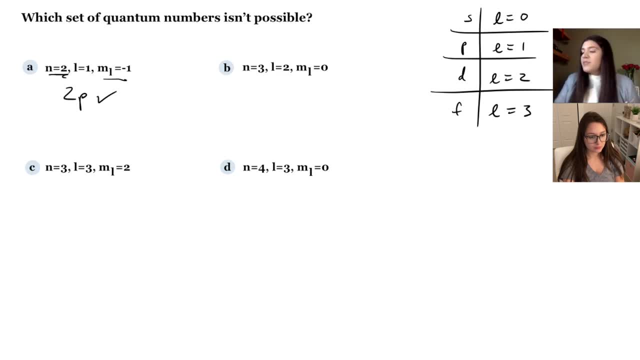 The next thing I'm going to look at is: I'm going to see: well, does the m sub l make sense that it's negative one? Is it allowed to be negative one? And the answer is yes, And it's because l is equal to one. m sub l is negative, l to positive l. And we're given, we're literally. 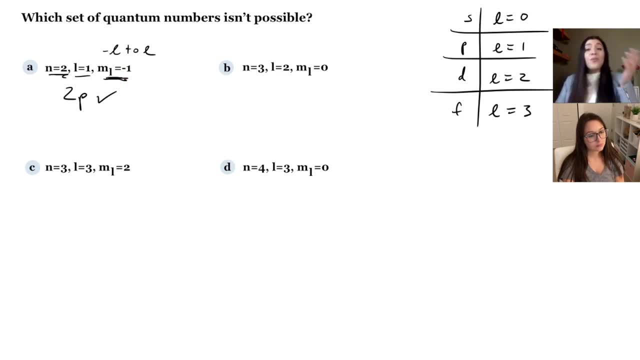 just given the negative l, That's fine. This didn't ask us for all the possible quantum numbers. It's just saying: is this specific set? is this specific set correct? So this one or isn't possible or whatnot, but this one specifically is correct, It works, It's valid. Does that make sense? 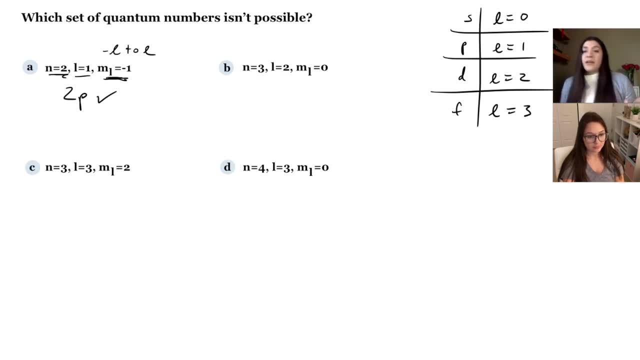 Yes, Okay. So then, looking at b, what would this be? So, once again, like this one was two p, what would this be? So this one would be three d. Okay, Is that allowed? Like looking at our periodic table. 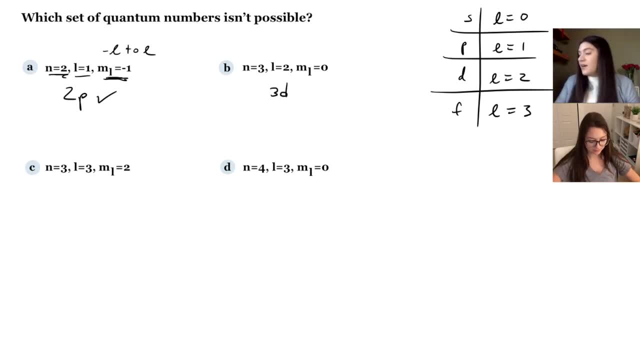 can we have three d? Yes, Does that exist? Yes, it does, So check. Next thing we look at is just the m sub l. So can m sub l be zero? Yes, Yes, Good, Because it would be negative two, negative one, zero one, two. 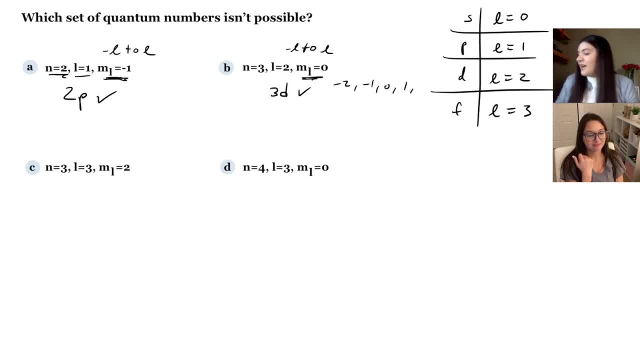 Exactly All of these, Exactly Perfect. Okay, So that one's fine. Looking at c, what would we have? We would have three f. Is that possible? Three f Exactly. So that reaction is perfect, because, no, we can't have that. 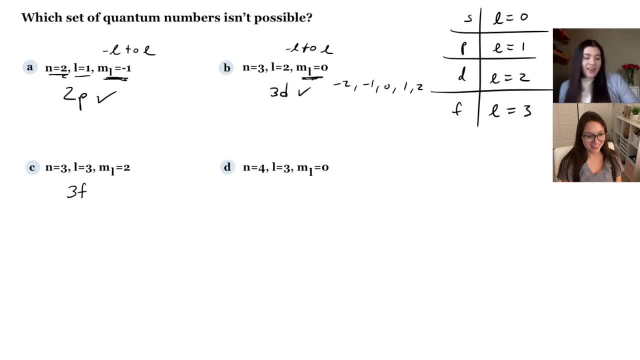 Okay, Yeah, No, I know. So, like looking at the periodic table, what's the lowest f that we have, like in the f block, Like what's the lowest coefficient or n-value? Well, it would technically be six, right. 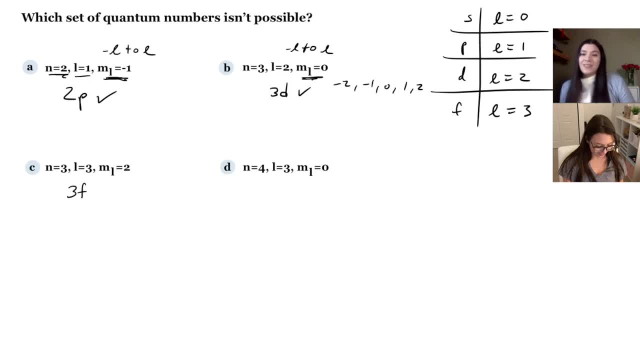 Try it again. Remember for f it's always two less than the row that it's in and the f is all the way at the bottom. It's the one detached from the periodic table or the main groups, So it's not six. 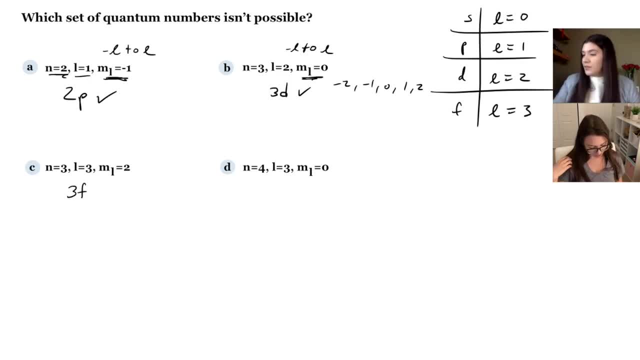 It would be four. So if I were to- Oh well, the reason I said six is because I was like bringing it back up to here. you know where you like take this whole section, Got it Okay? no, So we think of it like we would with the electroponfiguration. 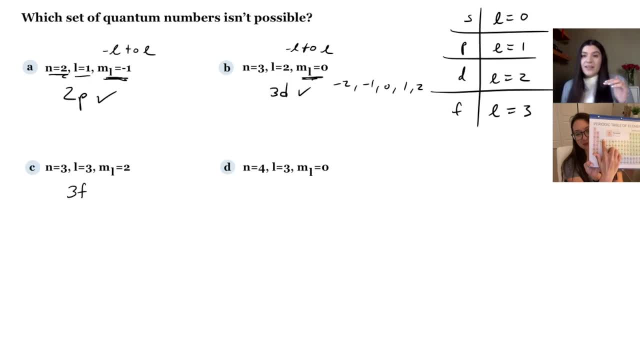 So we slide it up to where it would be, and then we take two from that. So it would have been six. so we take two from that and then four, make it four. Yes, Yes, Okay, Yes. 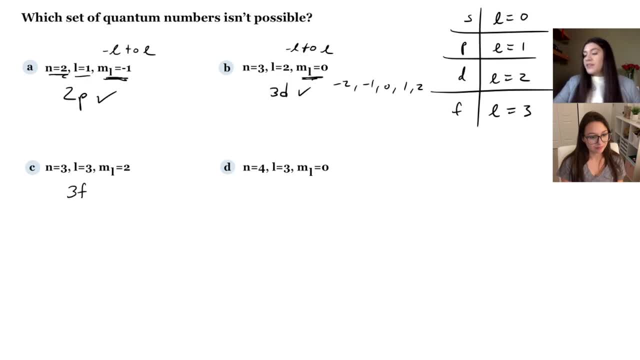 Cool, I forgot that one. So that's why this doesn't exist. It can't work because the lowest n value that we could have for f is four, So only four f and above. really it's only four f and five f exist, not three f. 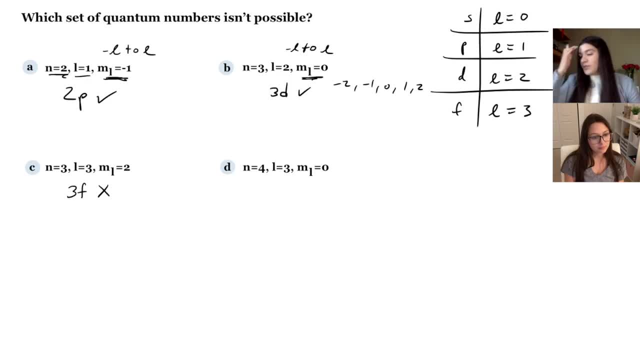 So that's why this is wrong. So for d, I mean we're still going to do d, just to you know, really make sure. but what would that be? It would be four f, And that's it. 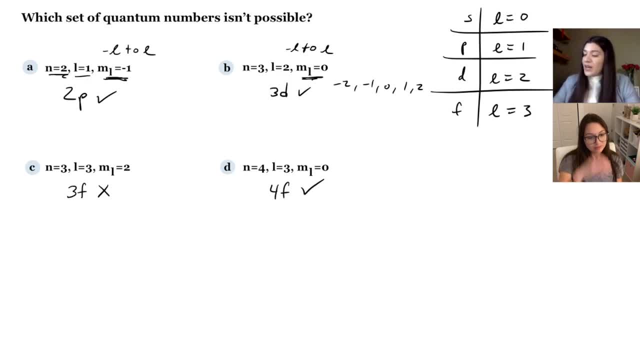 So, yeah, four f. we just saw that that's correct. That's why it works. We know that the m sub l can be zero, because what are all the possible m sub l values that we could get for this? one Negative, three negative, two negative, one zero. one, two, three.